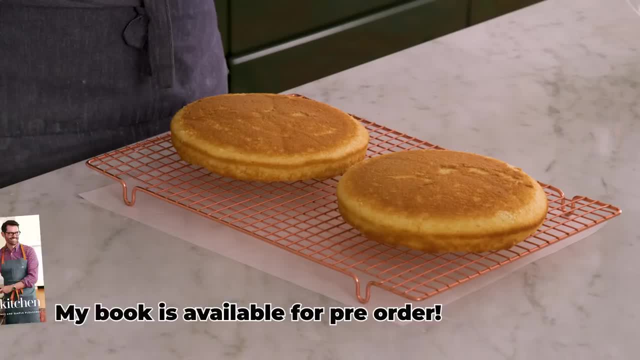 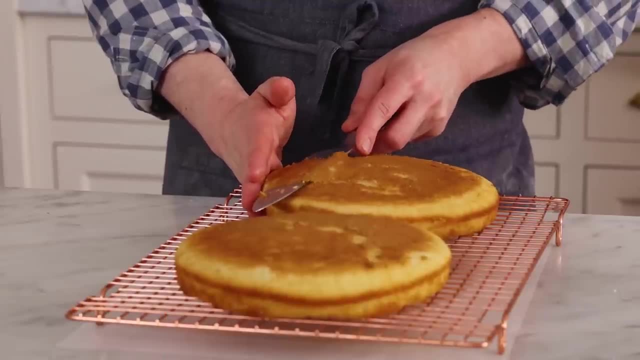 bits of over-caramelized or even burnt cake. So we're gonna give these layers a very, very gentle trim. You're also gonna find out that if you just crumble the cake in here and mix it with the buttercream, would it work. 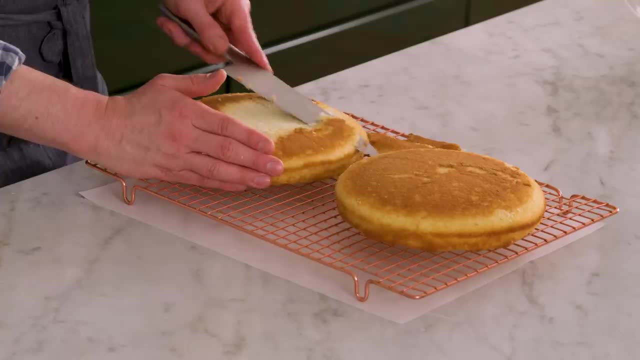 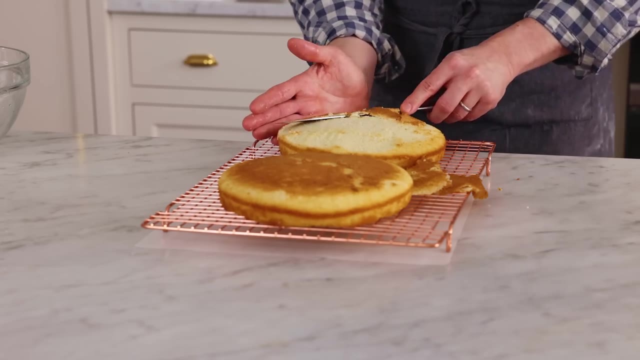 Pretty much. You'd have some issues which we'll talk about later, But oh my gosh, they'll look dirty inside, which is like disappointing, Because you want a cake pop to have like that nice, either light color if it's vanilla- 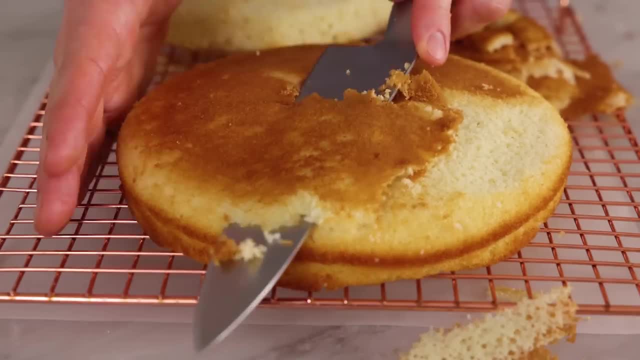 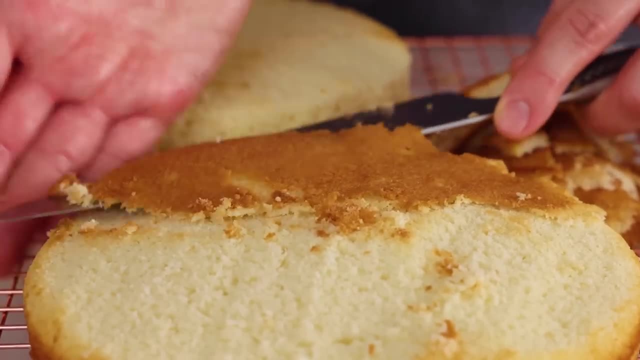 If it's chocolate, it's a totally different story. So I'm removing some of these caramelized sections And today I'm using two eight-inch cake rounds. It's probably even easier if you just made a big sheet cake. I'm also trimming the edge, which is a little bit firmer. 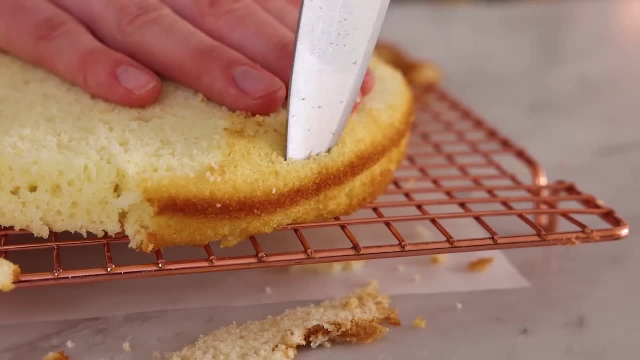 And what would happen is it would not mix in with the buttercream and you'd have not necessarily like a dry cake moment, but it would just be weird. Like you're like, hmm, what am I tasting right now? 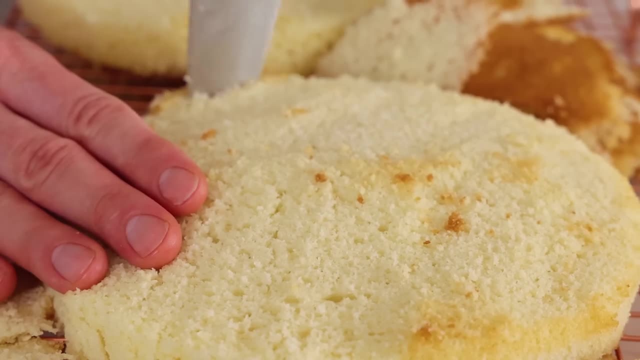 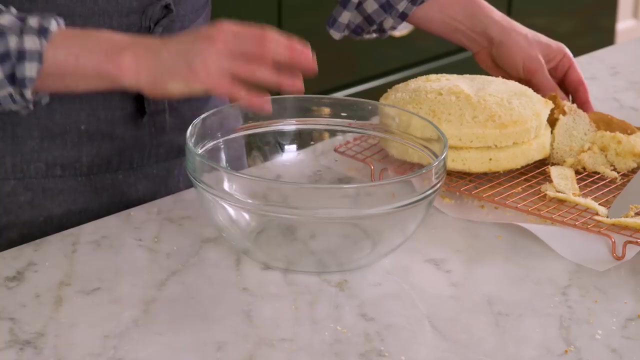 Is this okay? Whereas you want something to say: oh my gosh, this is delicious. throughout My cake's trimmed up. We're ready to go. Time to assemble. So grab a big bowl. You want a spatula? the frosting that works. 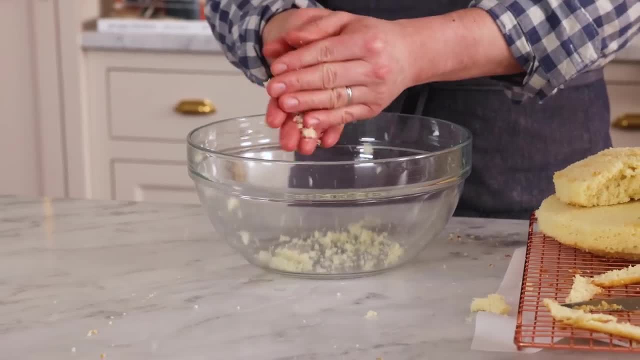 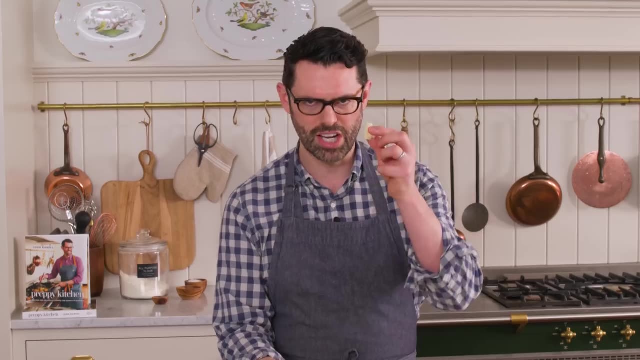 And you're gonna begin by crumbling up the cake. I wanna have little, uniform pieces, So just like in circular small motions, you can break it up. You don't wanna have a giant chunk of cake. It just creates problems of having a spongy texture. 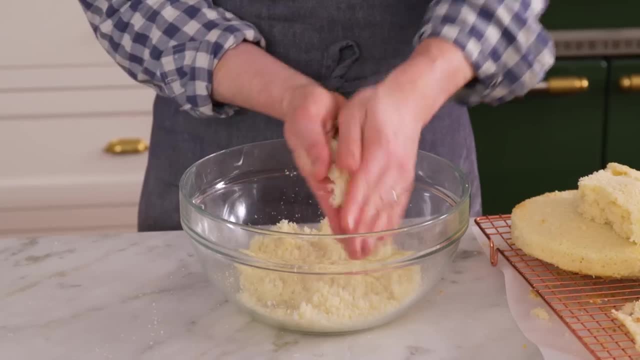 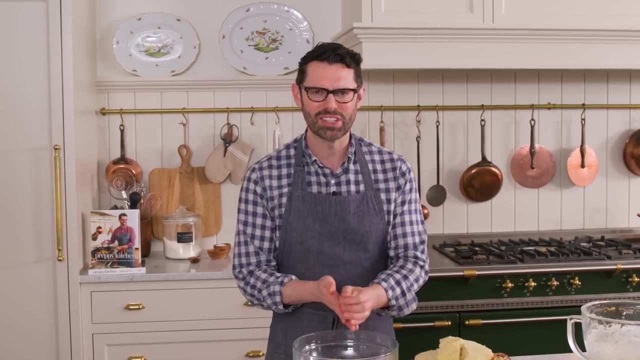 The deal with cake pops is you need them to be not firm, but they can't yield too much, Otherwise it just won't work. Things will crack, they'll fall apart and you'll be disappointed. You don't wanna be disappointed. 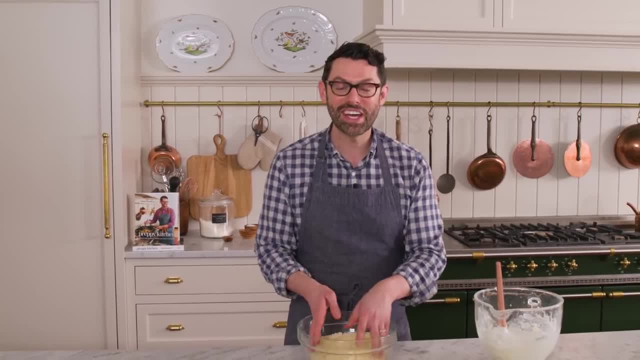 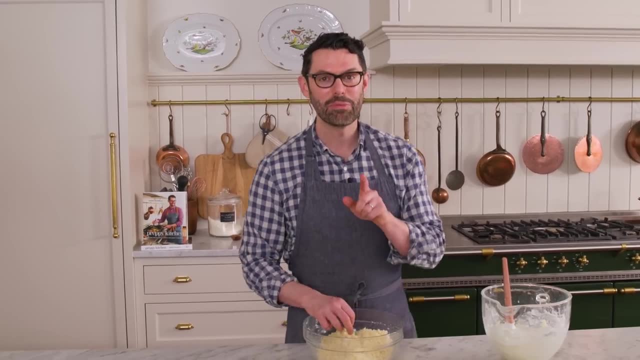 You wanna have a fun time in the kitchen? All right, Your cake is crumbled up. Give it one final look through. I swear these big clumps of cake are a problem, because what happens is we start adding our frosting in and using a spatula. 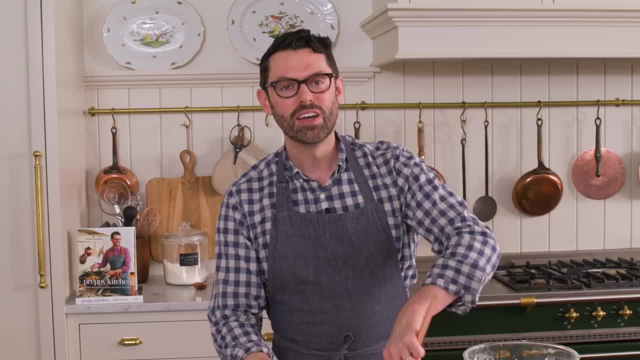 you could use an electric mixer if you want, but I don't wanna overmix this. You should have a consistency similar to wet sand, but it shouldn't be like a paste. You wanna have a little bit of the cakey texture like. 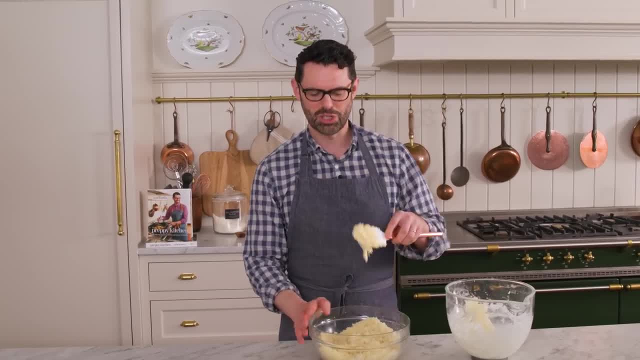 but it shouldn't be like a paste. You wanna have a little bit of the cakey texture, like, but it shouldn't be like a paste. So right now I'm using my spatula and I'm tossing it around and smoothing it through. 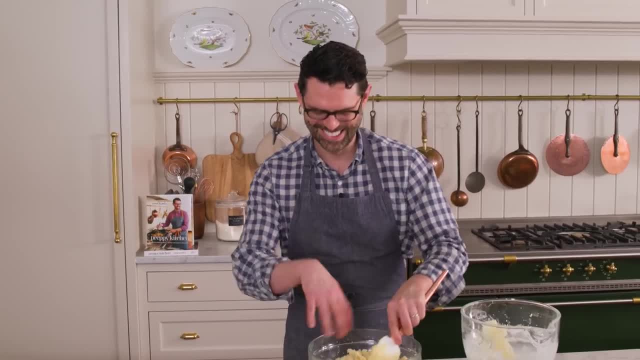 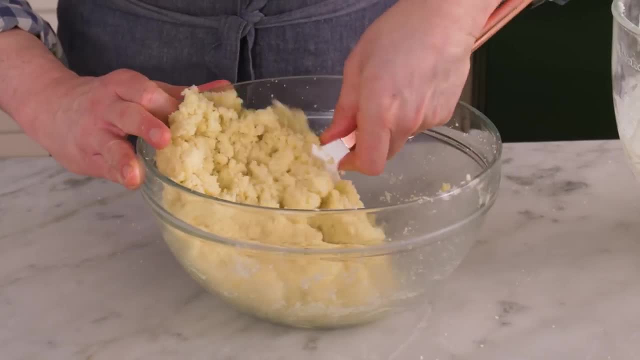 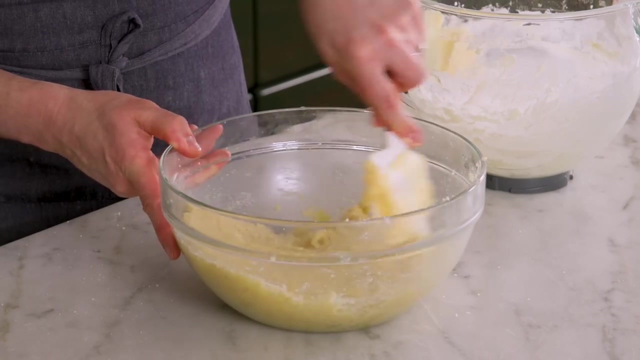 So it's like I'm a cat pawing at the bowl. If there's any places where it's dry like you see here, those cake balls won't hold together and you're not gonna be happy, I promise. Okay, So now you can see wet sand mixture. 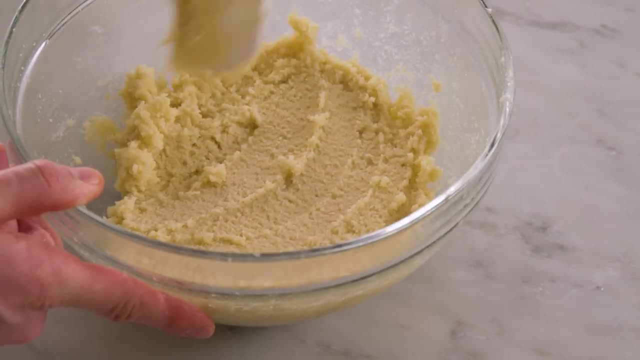 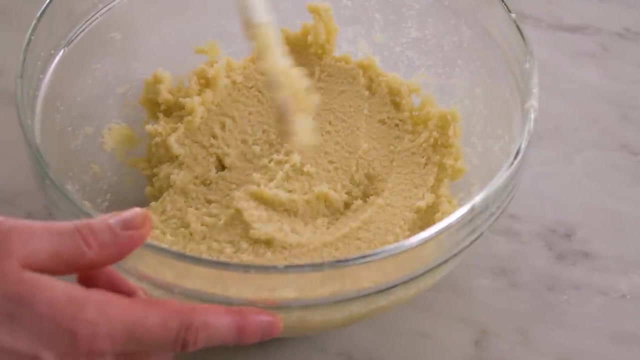 Look how homogenous it looks. all the same, throughout I don't see any giant balls of cake hanging out. There's no clumps of frosting and you can see it's still delicate, So it's pulling apart. There's cake in there. 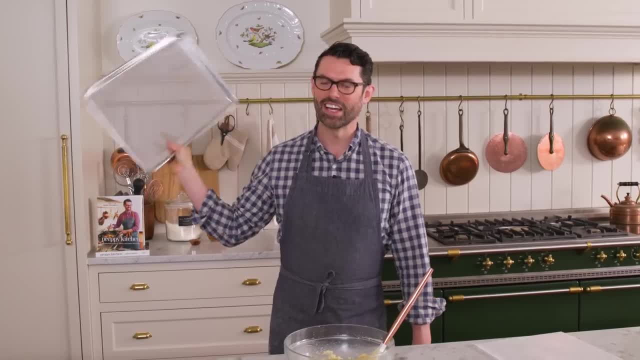 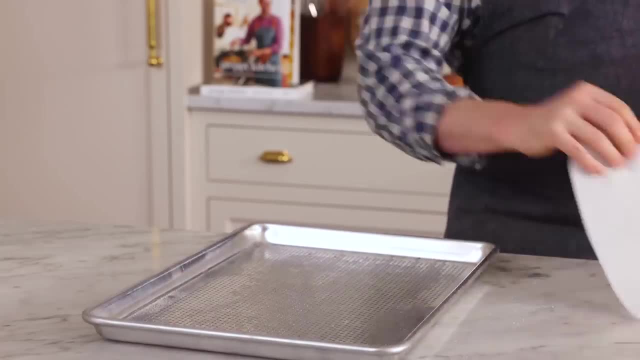 This is ready to roll, It's time to grab a baking sheet. This is a special one, but we're not baking, So it doesn't matter. Little parchment paper to keep things nice and clean. I want about one to one and a half inch. 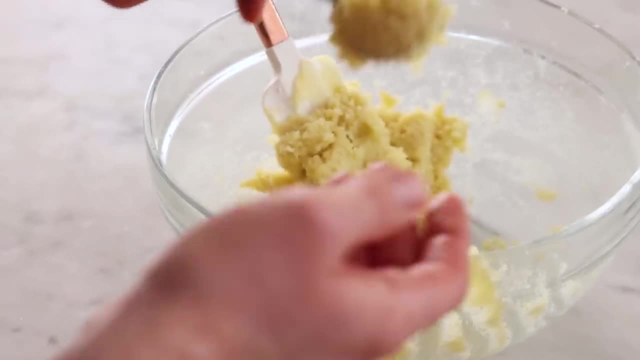 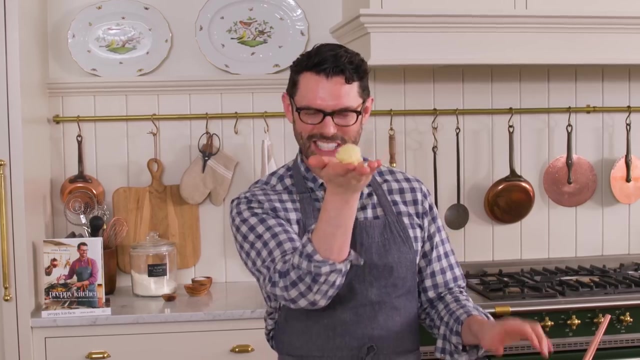 I like mine a little bit larger, So I'm using a one and a half inch scoop. You're gonna roll these and it's gonna be okay. They will not look like perfect spheres, but you can fix this later, because we're going to chill them. 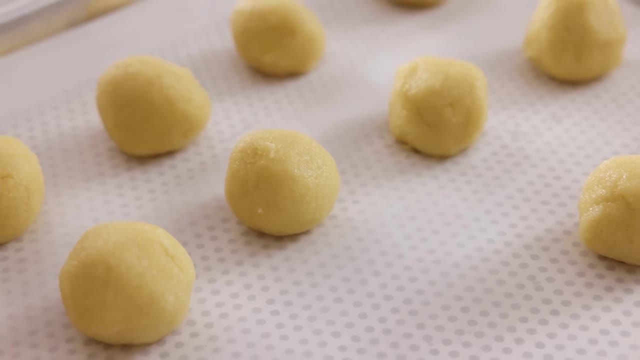 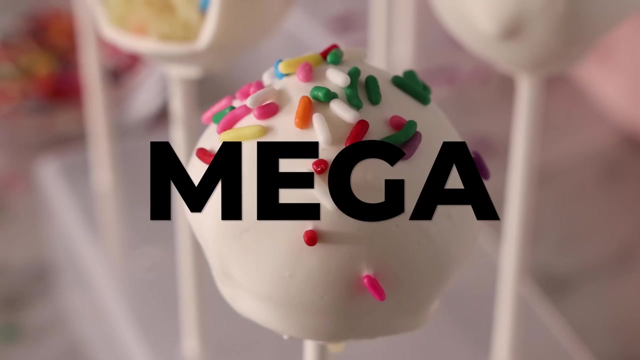 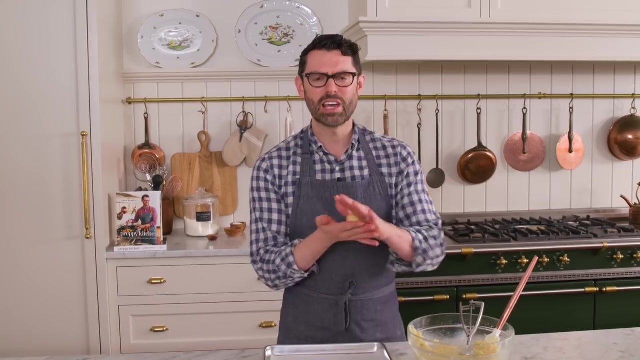 For all my fellow Virgos out there and everybody else. these guys are about 35 ounces, 35 grams. They're 35 grams Mega cake pop. So right now they are so soft. They've been through a lot, These cake pops. 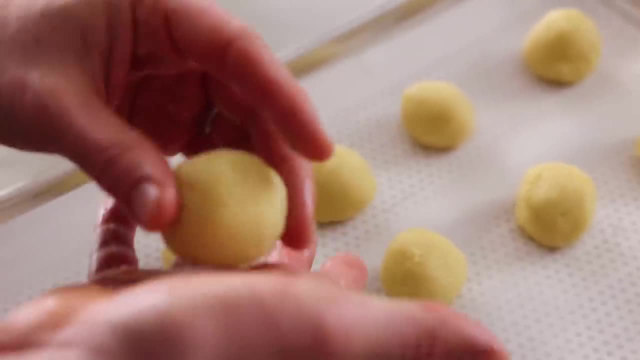 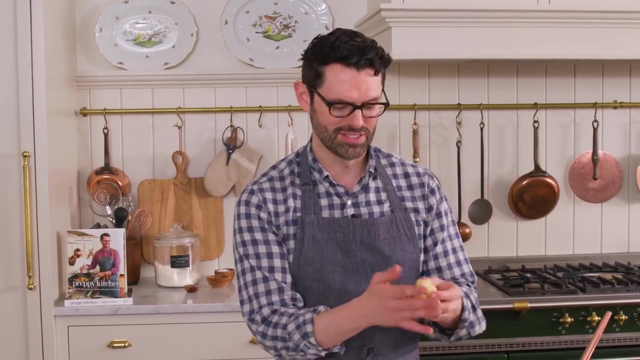 are gonna firm up when we chill them up And after they're chilled we can give them a final roll to get them to be a little bit prettier and less lopsided, if that bothers you. These guys are looking great. I'm loving that light uniform color I got. 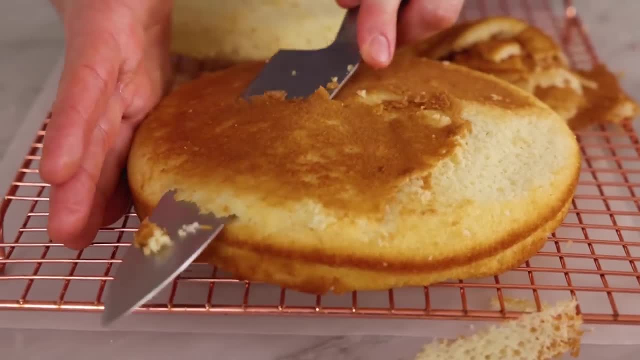 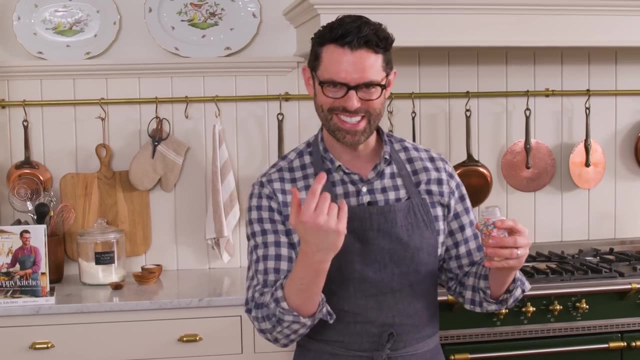 from just shaving away a little bit of caramelization on the outside. I am, however, wanting to add some more color here, So now I'm just gonna add a couple of tablespoons of sprinkles. Look how pretty this is. Come here. 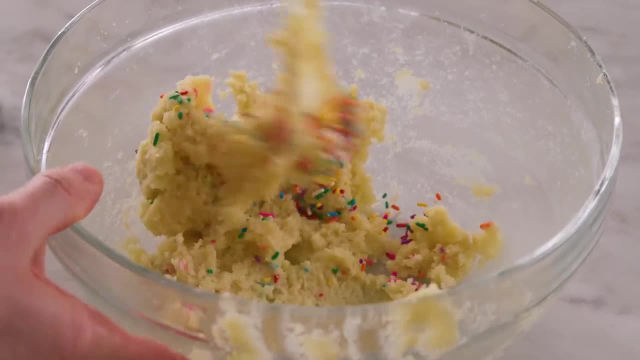 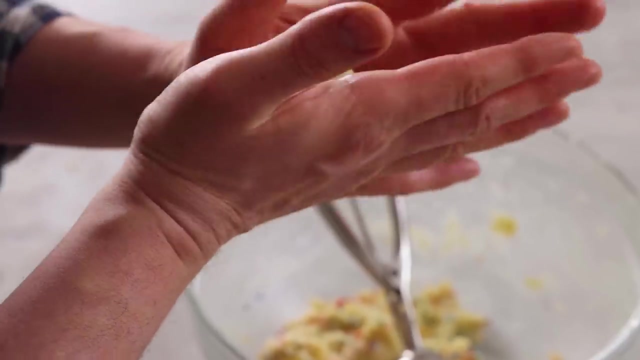 Now we're just gonna mix that in So they're uniformly distributed, And just like that. look how much better that is. I kind of like the sprinkles situation even more, So now, when you bite into them, you'll get a colorful little surprise. 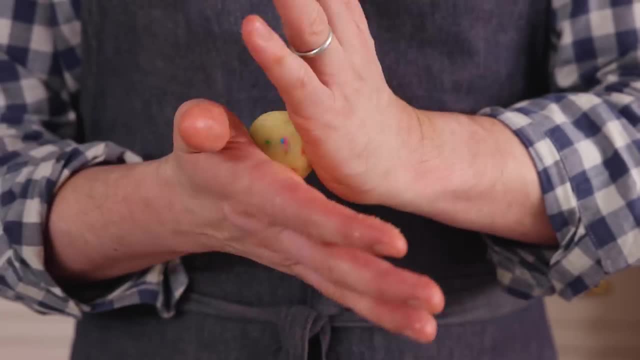 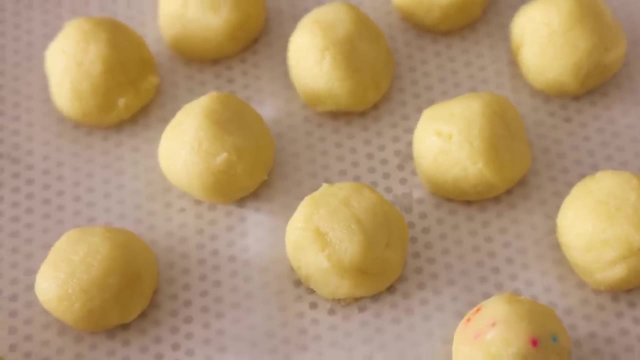 Isn't that nice. You know, on the channel we have how to make sprinkles and it's so fun. My last cake ball is rolled. These guys are gonna go into the fridge for four hours or into the freezer for half an hour. 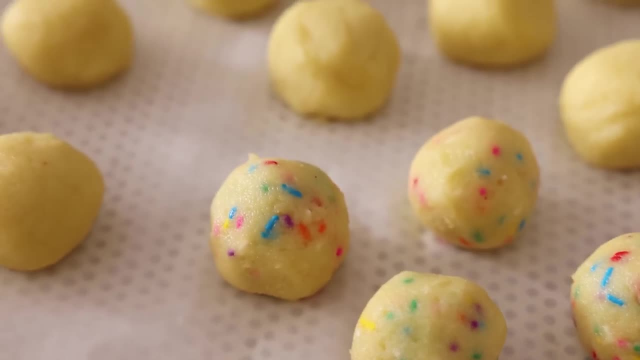 That's what I'm gonna do. Towards the end of your chill time, pull those cakes. Towards the end of your chill time, pull those cakes Once your cake pops out and you can see they look a little misshapen. 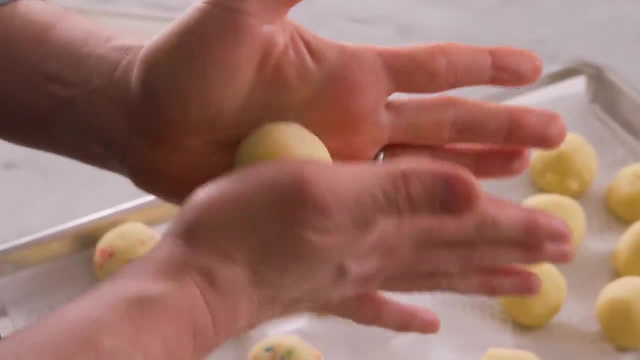 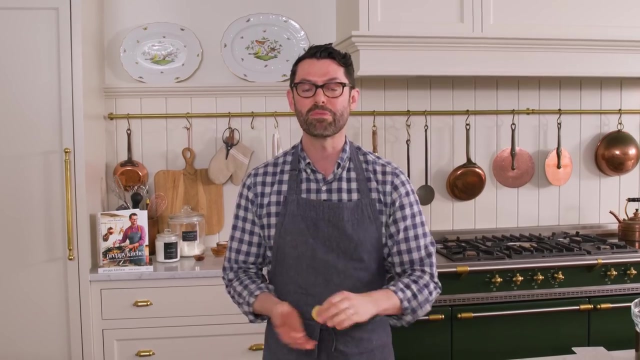 not quite right. So what we're gonna do is give them a quick roll. Now they feel so much firmer, which is great. Once your cake balls are nice and round, we can pop those back into the freezer while we work on our coating, which is a whole situation. 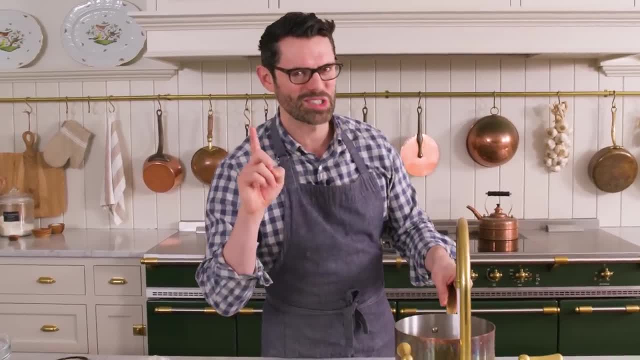 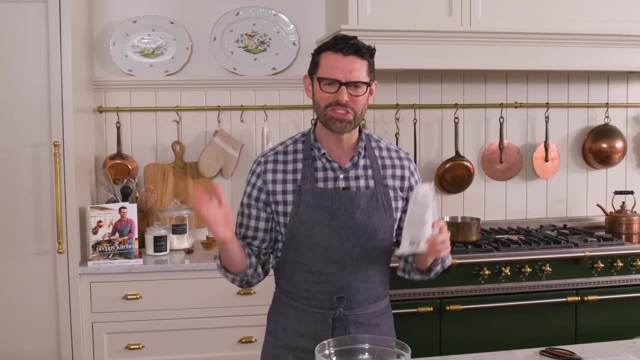 So I have to talk to you about it. I'm using a double boiler and I'm gonna explain why I'm using chocolate melting wafers. If you wanna use chocolate, I am so proud of you. Good job, they'll taste delicious. 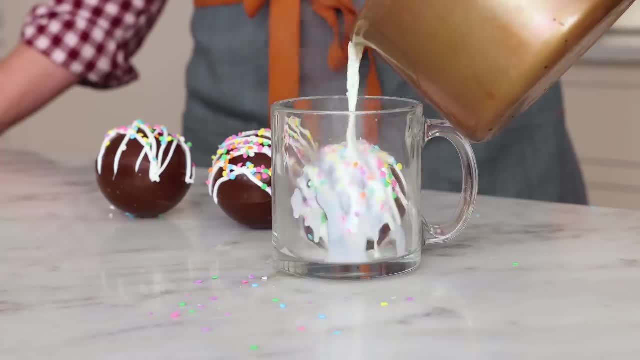 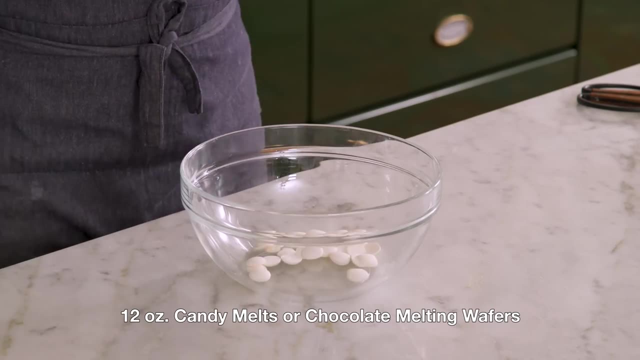 but it's rather finicky because if you've watched my hot chocolate bomb video, you know tempering chocolate is not the easiest thing in the world. Chocolate melting wafers, however, are not based with cocoa butter, so you can melt them really easily in the microwave. 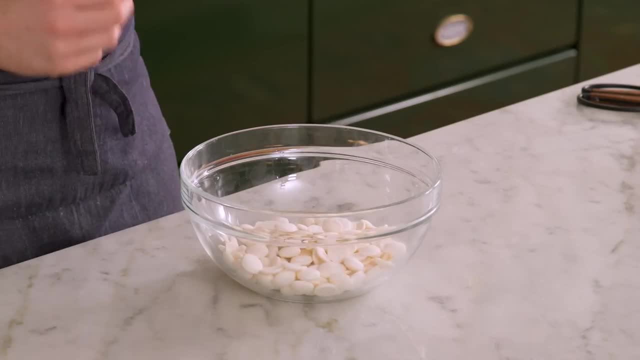 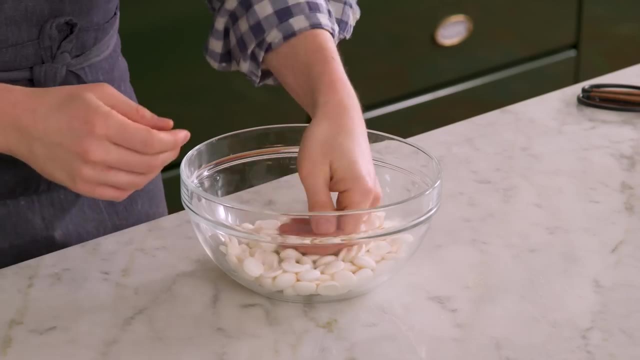 or so I've been told. In truth, they're actually a little finicky themselves. They tend to kind of just like not melt a lot of the time, depending on the batch you get. So I'm using a double boiler, plopping them onto my simmering water. 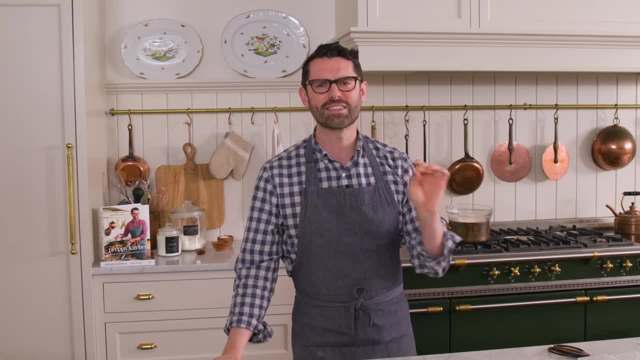 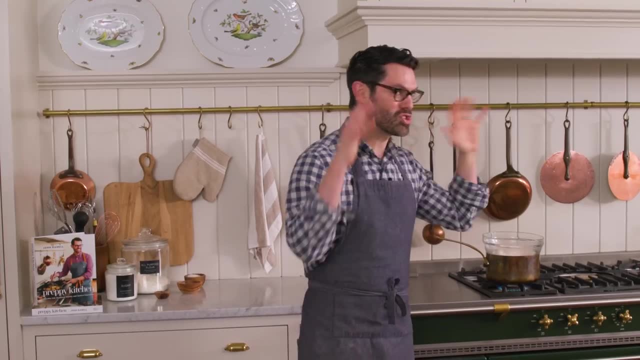 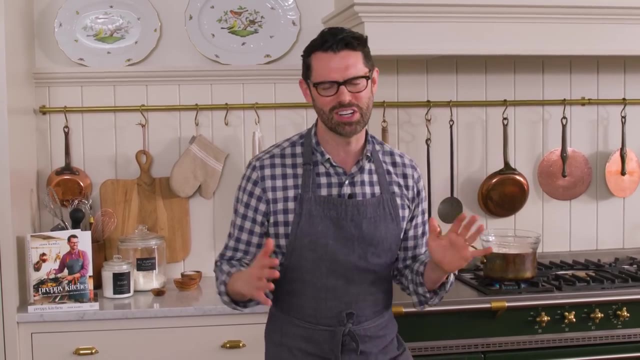 I'll be stirring. occasionally, These guys are so much less likely to burn. It's amazing, but I swear. in the microwave what happens is your bowl gets so hot and then the candy melts are fairly cold on the inside and you're just left with a frustrating situation. 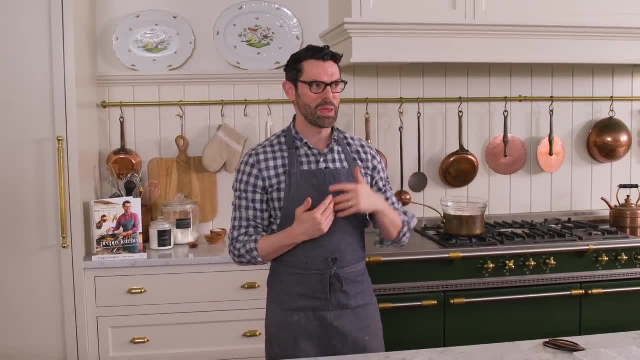 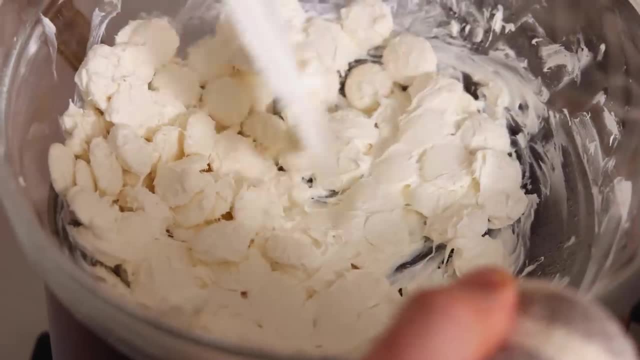 So my suggestion to you, having learned the hard way many times, is to just melt these in a double boiler, and it should be easier. We'll find out. Candy melts also have the advantage of being really white If you compare them to white chocolate. 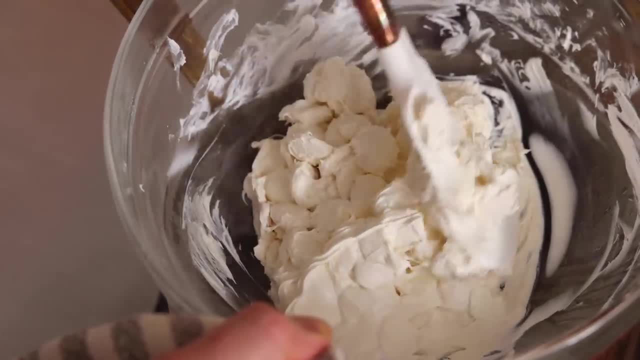 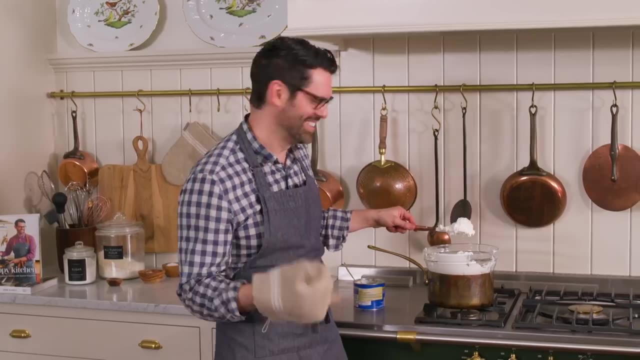 white chocolate is actually a light yellow color which people don't realize until they see it on their cake pop and they start asking questions. So my candy melt is melted, but, as you can see, this doesn't look very dippable, does it? 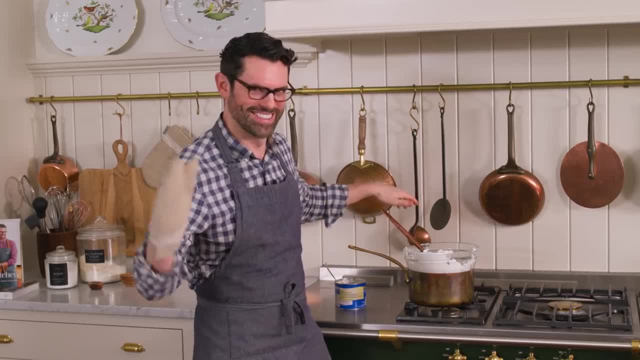 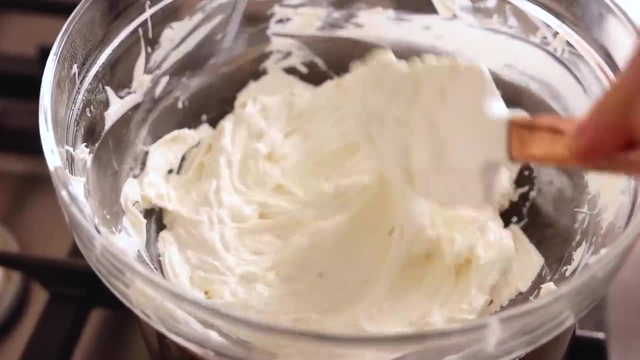 It's fairly thick, which happens a lot of the time, So I'm gonna add a teaspoon or so of shortening right in there. You could use coconut oil as well, as long as it's not the fractionated kind. It needs to be a solid at room temperature. 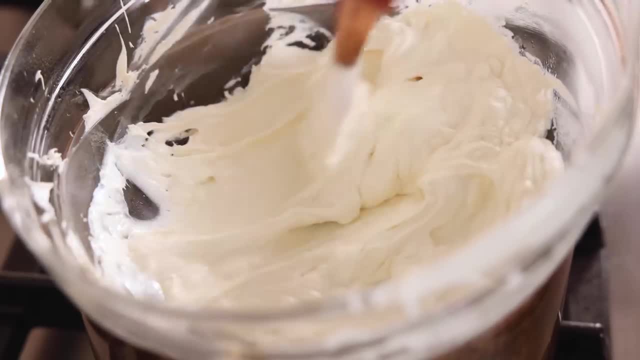 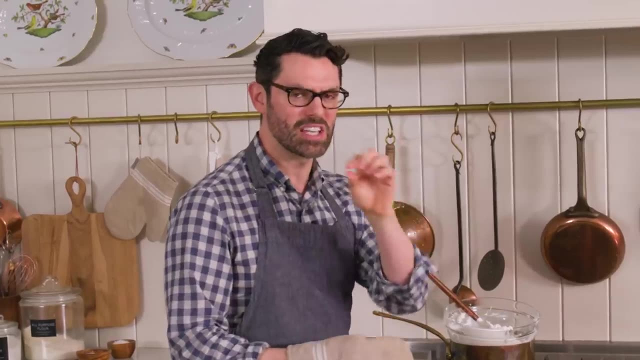 And you're gonna mix that in really well. You'll see an immediate change in the texture because it needs to be able to be dippable. but you need to mix it in well because if there's a streak of coconut oil, that will not set up and it'll be a cracking point. 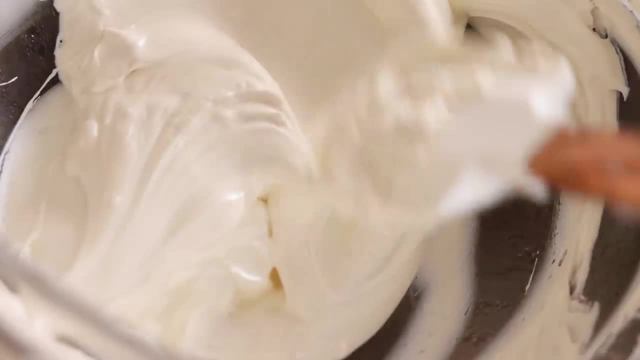 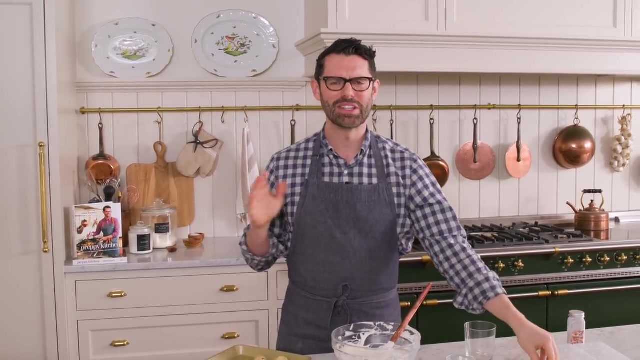 See how it's falling off of my spatula. now That means we're ready to dip. Let's get it Ready to dip in. A couple things are gonna happen together at the same time. It's gonna be amazing One: I grabbed a batch of my cold balls of cake. 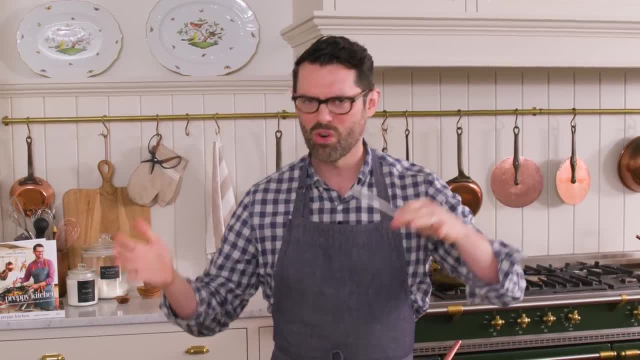 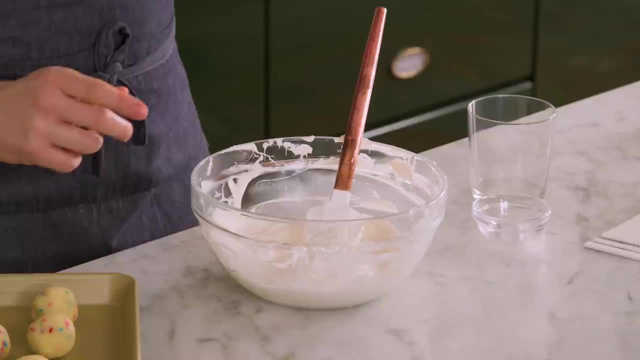 out of the freezer. We're working in batches because when things get warm you get sad. Now I'm gonna take my little treat- sticks, as they're called- dip the end in chocolate and then actually I'm gonna make a little hole. 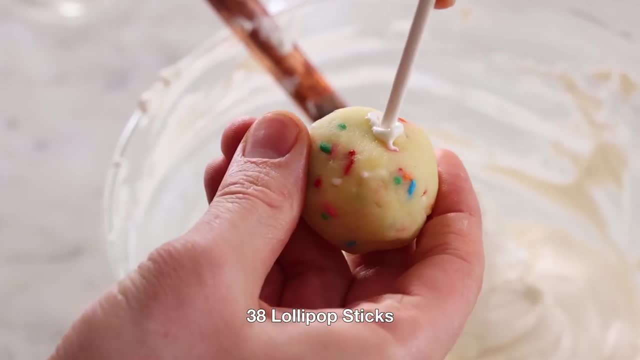 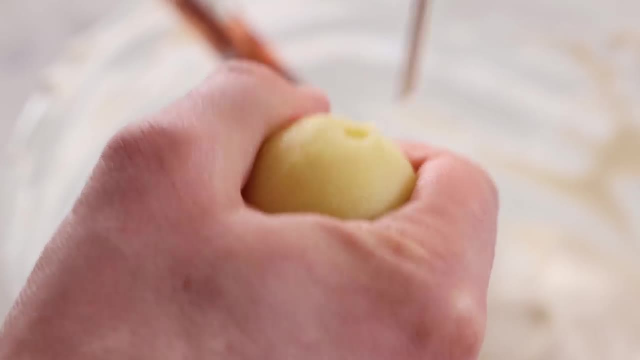 and then dip that in chocolate like this And this will be the glue that kind of helps hold it in. The sticks shouldn't go too far in because you don't want them coming out the other side, but you need to have a good base to hold on. 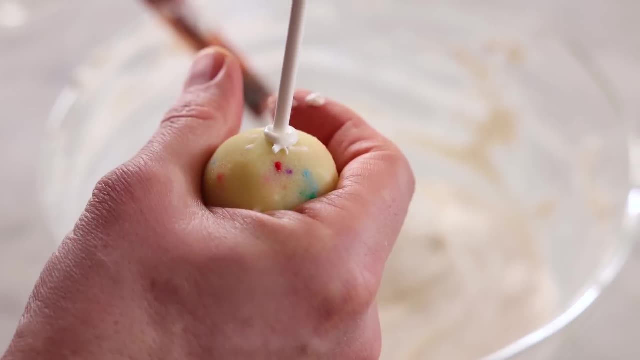 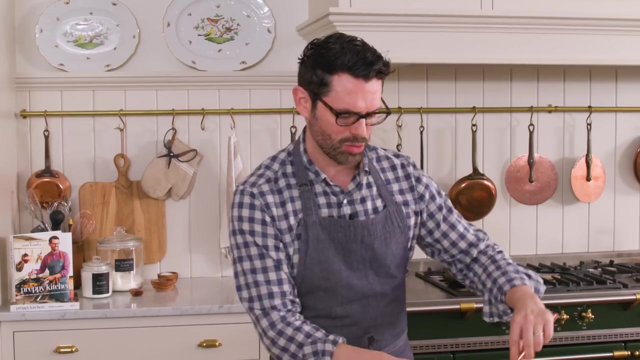 for our crucial dipping step. Are we ready to dip? No, we are not ready to dip. That would be bad, because one it's a bit awkward to dip into the bowl, so I will be transferring my chocolate melting wafers. 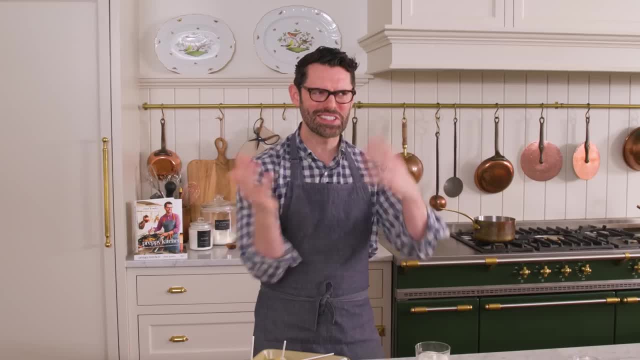 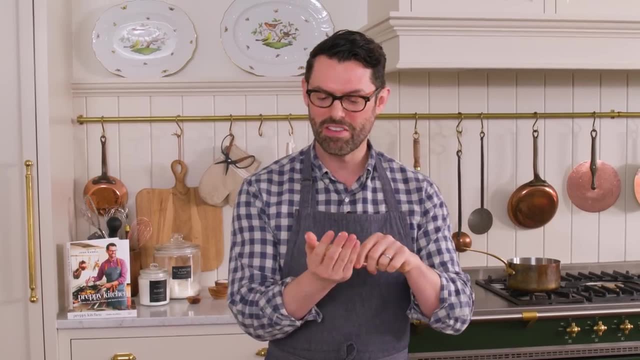 that I've melted into a cup. Also, there is some science here, because these guys are cold. now This is fairly warm. What'll happen is, if these are too cold and you dip them in this hot candy melt will harden over this cold ball.